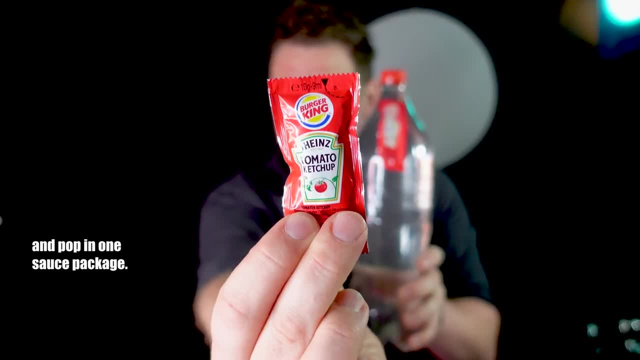 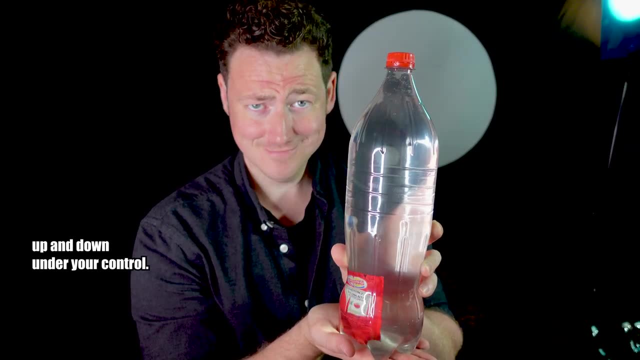 Get an empty bottle, fill it with water and pop in one sauce packet. Now give it a good squeeze And the ketchup packet seems to dance around Up and down under your control. The more you squeeze, the lower it goes, and if you keep going, you can find a sweet spot in the middle. 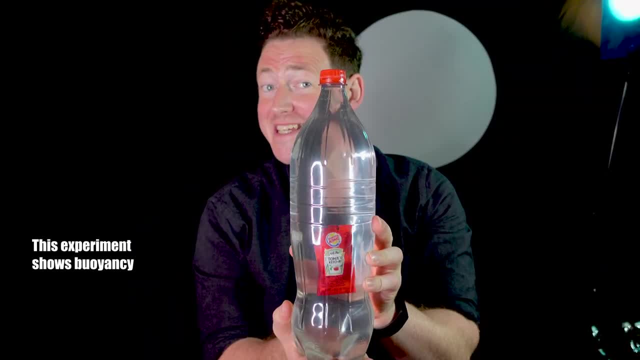 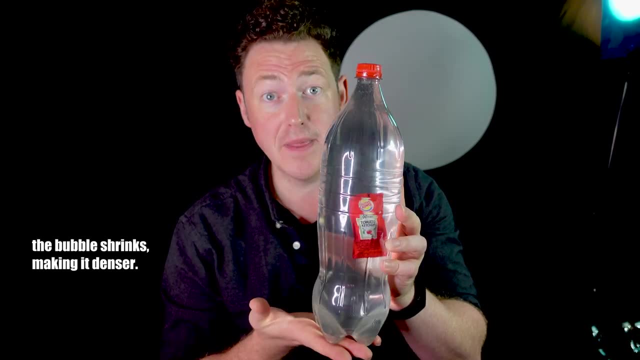 Now, why does this work? This experiment shows buoyancy and density in action. The ketchup has a tiny bubble that keeps floating, and when you squeeze the sides of the bottle, the bubble shrinks, making it denser, and that's why it sinks to the bottom. Release the pressure. 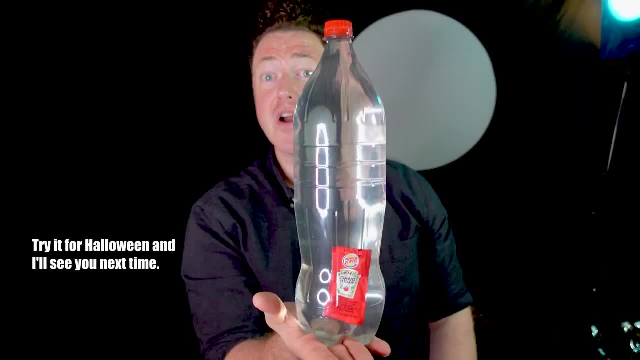 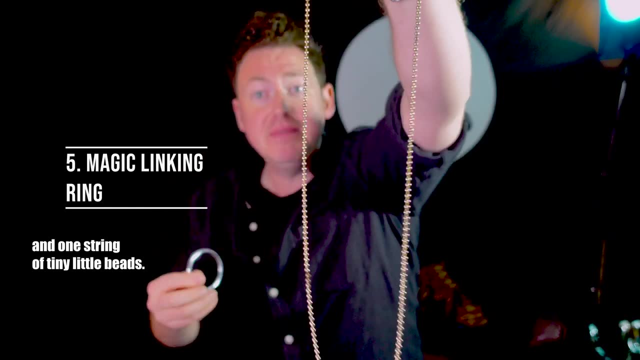 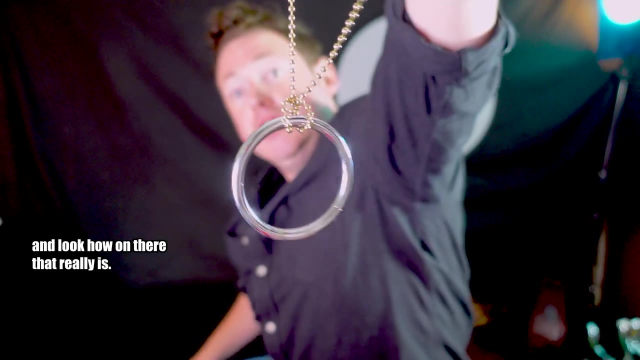 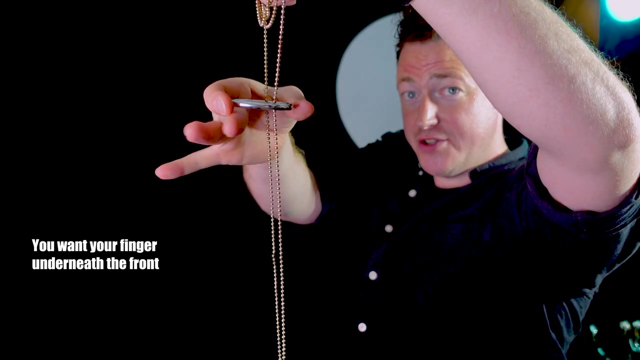 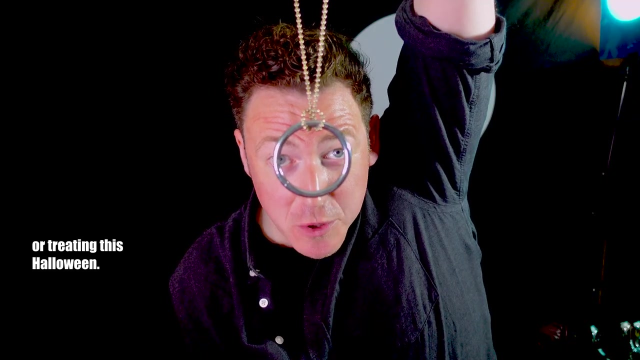 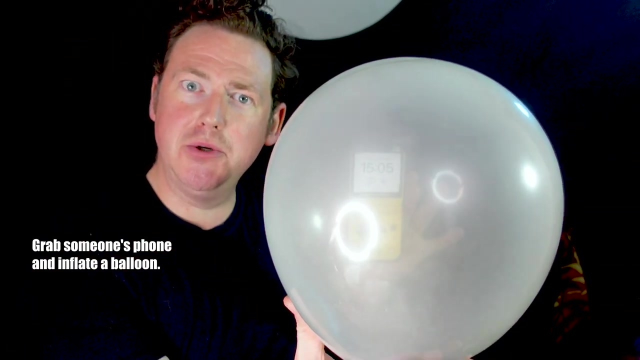 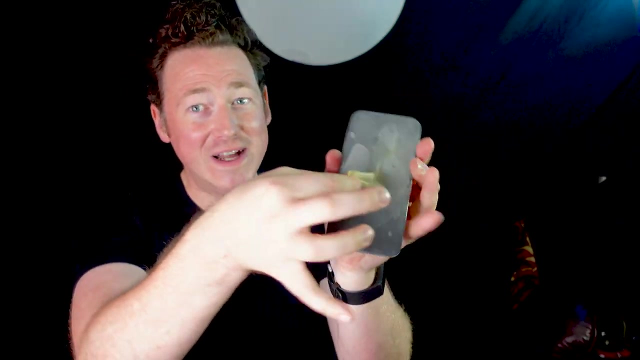 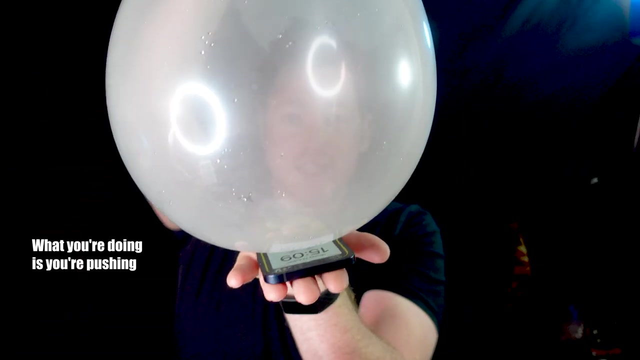 and the bubble becomes less dense and it floats to the top. Try it for Halloween and I'll see you next time. Grab someone's phone and inflate a balloon, and now you're gonna put your phone inside a balloon. All the way inside. you can even see that the screen still works. What you're doing is you're. 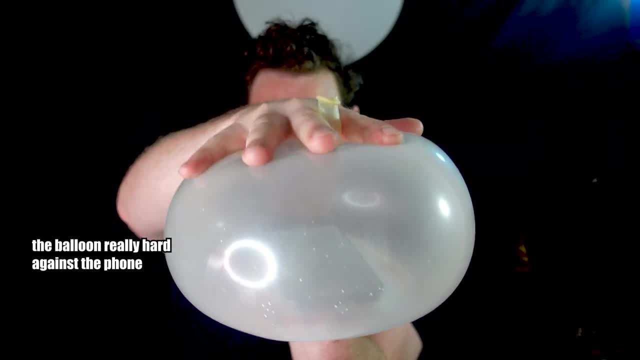 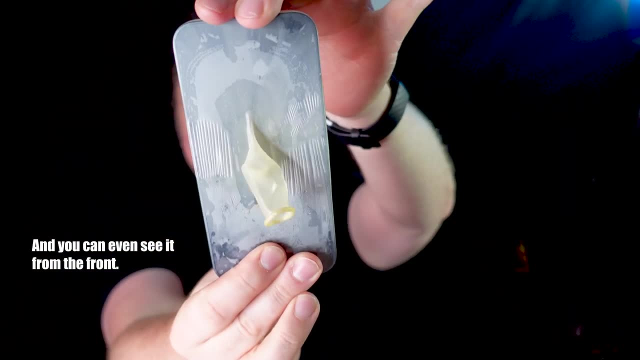 pushing the balloon really hard against the phone and the phone sinks into the balloon, just like that. That's what it looks like, and you can even see it from the front, but from the back you can tell it's not going all the way through, it's just gone round, and that is how to get your 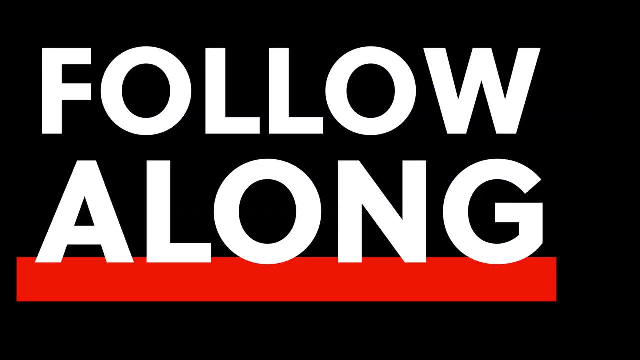 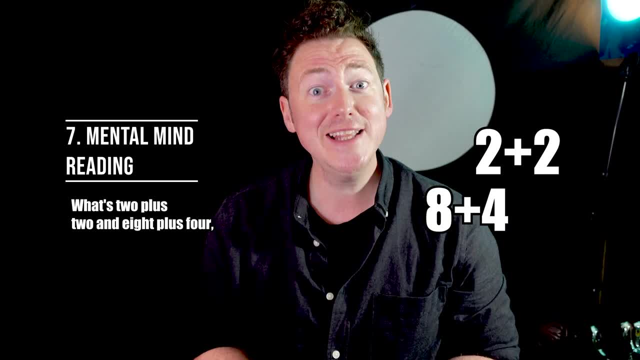 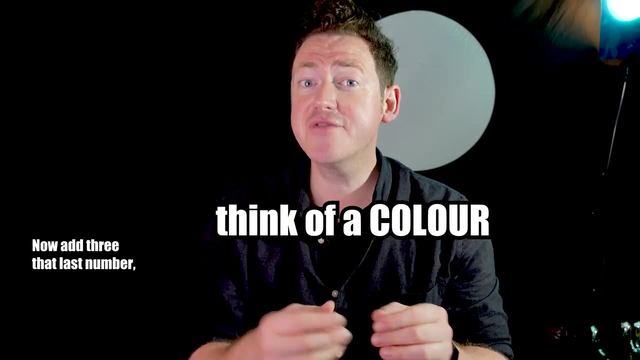 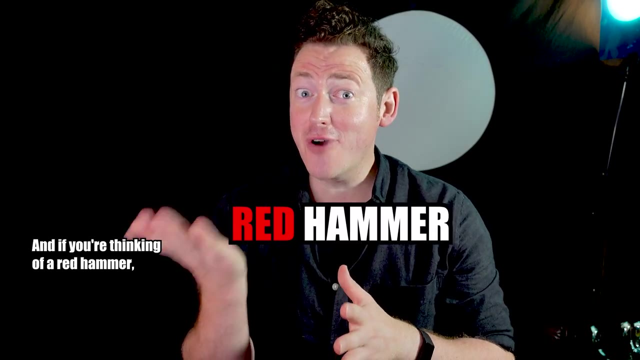 phone inside a balloon. Quick maths time: What's 2 plus 2? An? 8 plus 4? 9 plus 27? Now add 3 to that last number. Think of a colour, and now of a tool. Double tap the screen to lock it in. and if you're thinking of a red hammer, then I successfully read your mind.